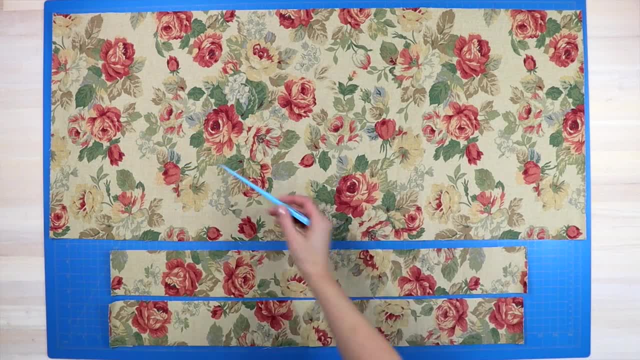 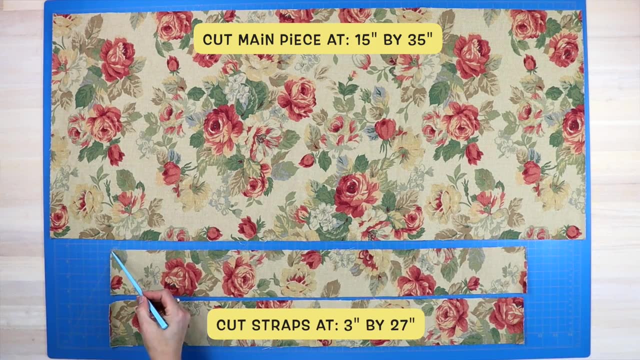 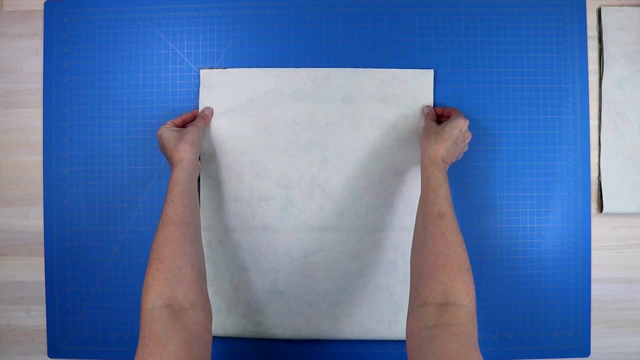 All right, let's jump on in. Cut your main piece of fabric at 15 inches by 35 inches and then two straps will be cut at three inches by 27 inches. Take the main piece of fabric and fold it right sides together so the inside lining is facing out. Line up those side edges, clip them in. 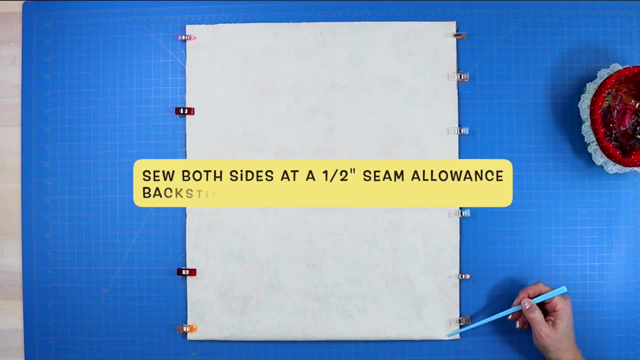 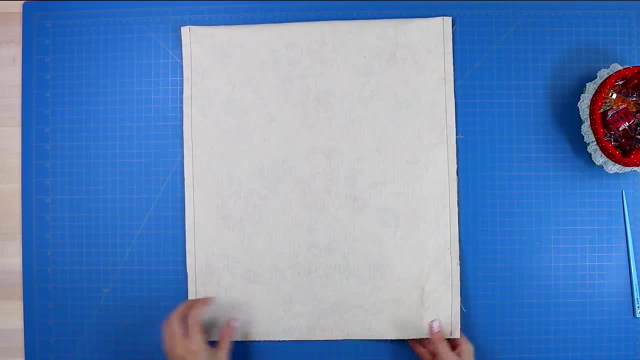 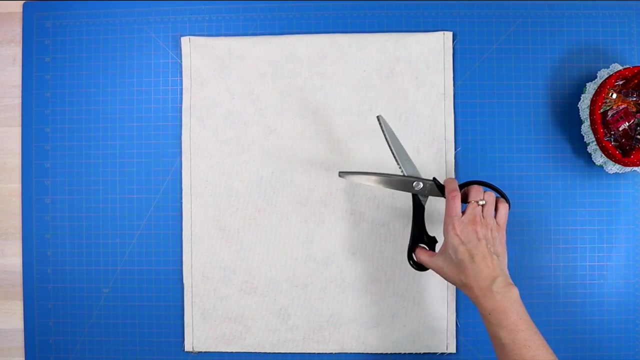 place and then sew a half inch seam along both side edges. You will start and stop with a back stitch. This next step can be done two different ways. One way is you can use a pair of pinking shears and you can snip along both of your raw edges where you just sewed your half inch seam. 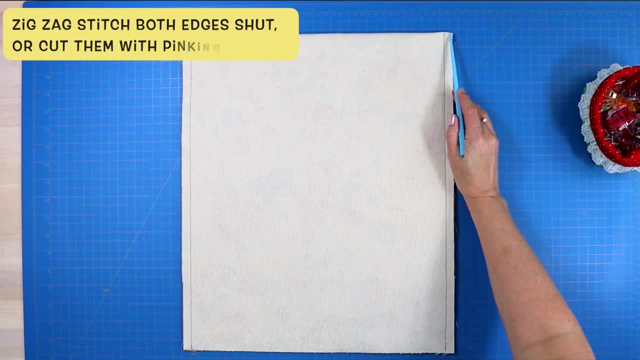 allowance and that will stop your fabric from fraying. But because we don't have a lining to this fabric, I actually recommend sewing a zigzag stitch So that you can see how the fabric is going down. both of these side seams Again start and stop. 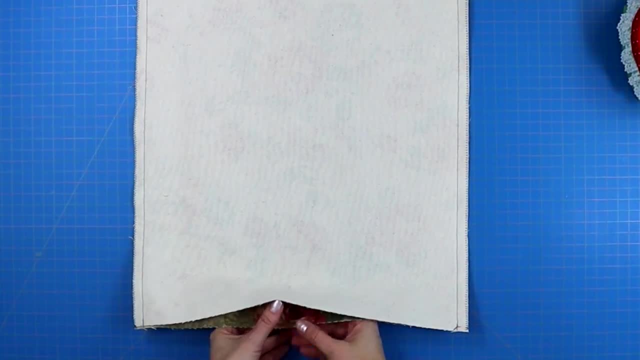 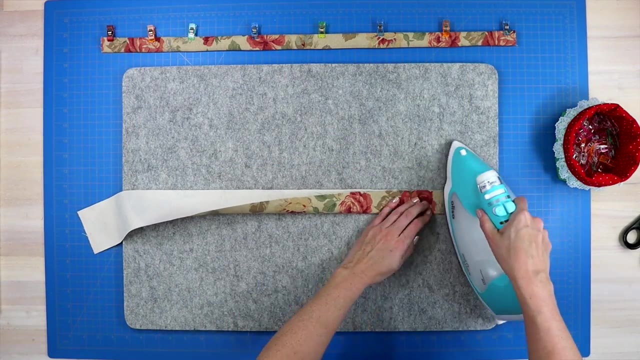 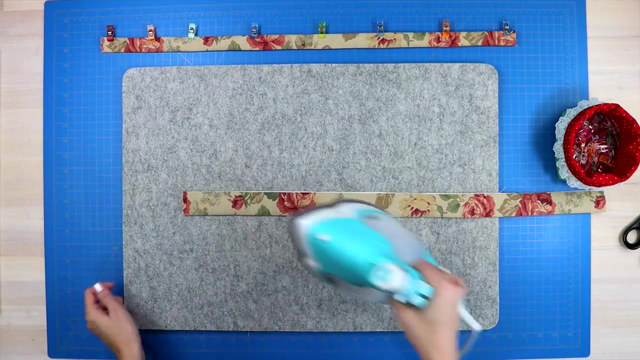 with a back stitch. And this is what it looks like, with that zigzag stitch along both side seams. Now it's time to get our handles ready To prepare your straps. you will fold your strap in half, wrong sides facing in, and then just press it so that you have a nice center crease. Once you've. 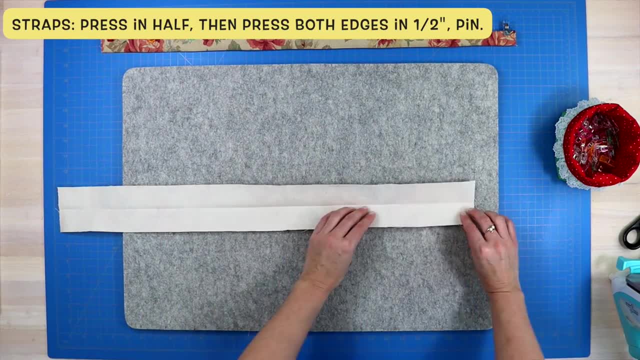 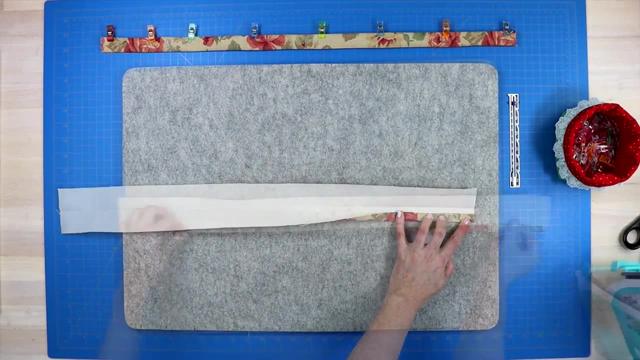 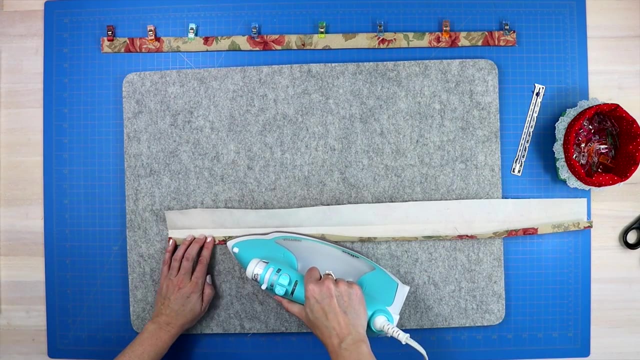 done that, then both long edges need to be folded in a half an inch towards that center crease. So that's going to be our center fold. As I'm pressing this half inch crease all the way along, I will check on it with my measuring gauge to make sure that it is a half an inch all the way across. 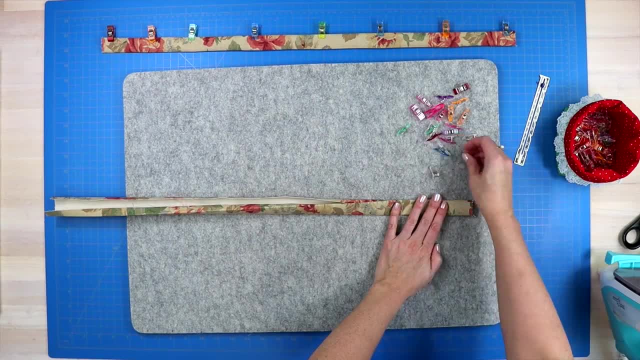 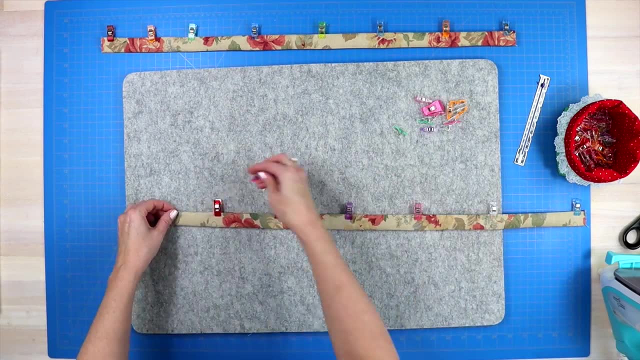 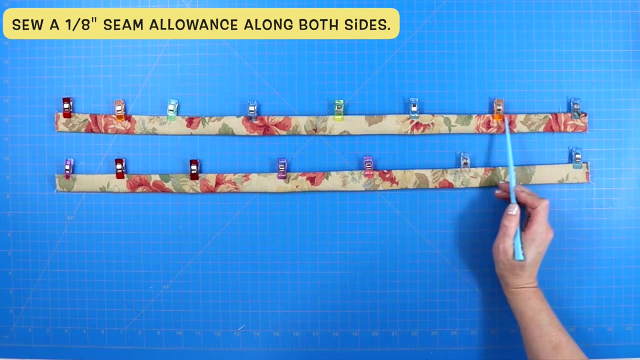 Do this, of course, on both sides, and then you can fold your strap in half once again, lining up those two outer edges and clipping it in place. Now we will sew a seam along that open edge first. So start with a back stitch, then sew an eighth of an inch seam allowance. 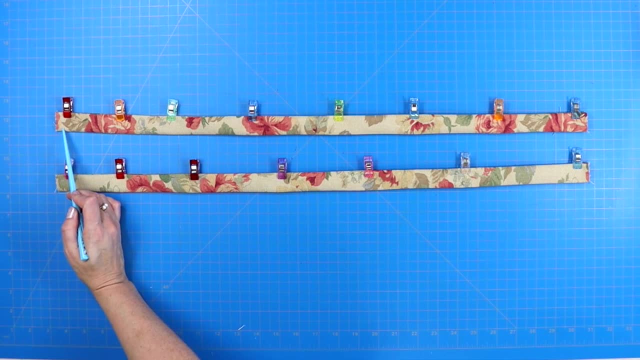 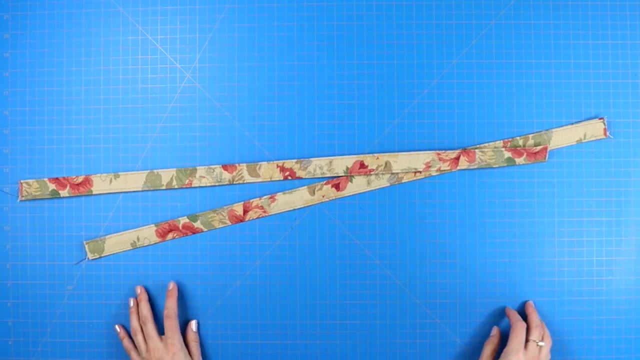 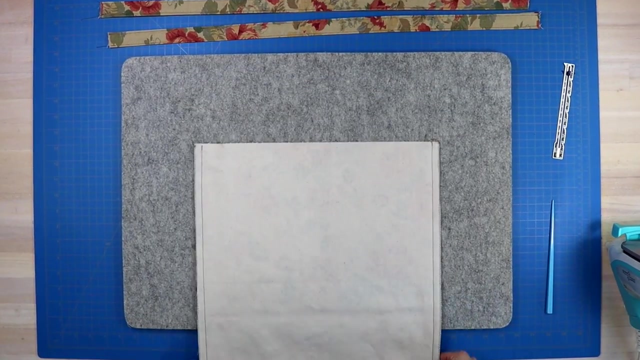 Along that edge, then just pivot down to the other corner and sew that eighth of an inch seam allowance again along that side, and then stop with a back stitch, And this is how your finished straps will look. once you've finished those seams, Now we need to attach our straps to our tote bag. 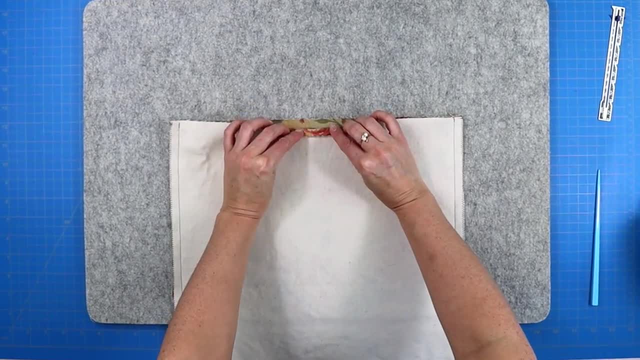 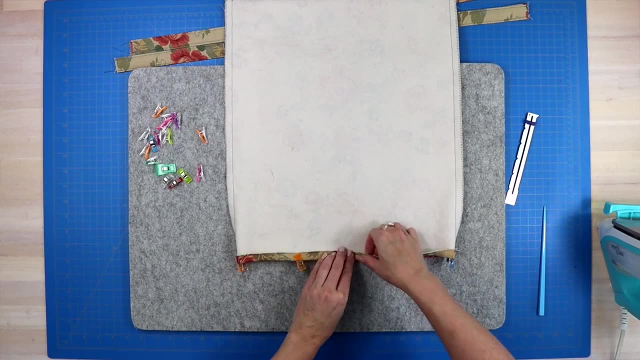 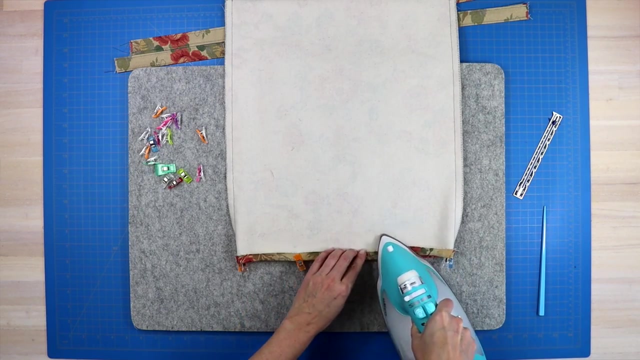 So find the opening of your tote bag and press the entire top edge down a half of an inch. Now I'm doing this on my wool pressing mat because this is where it's easiest for me to film, But I do recommend just doing this on a normal ironing board, because then you'll be able to. 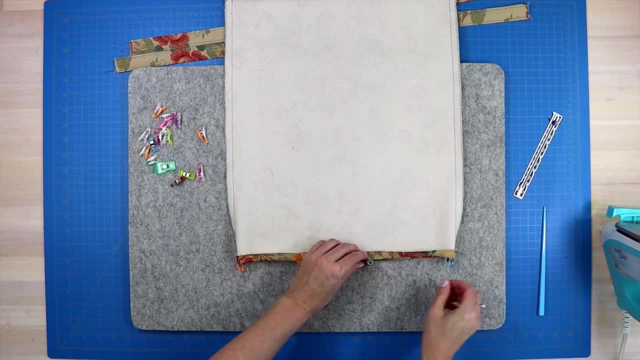 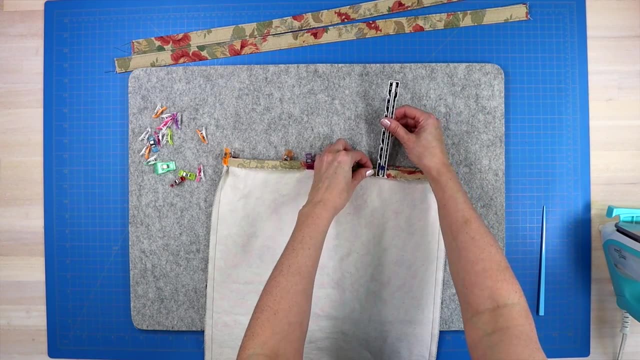 just wrap it around that outer edge and then pressing the seam will actually be quite easy. So press that seam in a half an inch and of course check on it with your measuring gauge, And then I just grab my clips and clip it in place so that it can cool folded down. 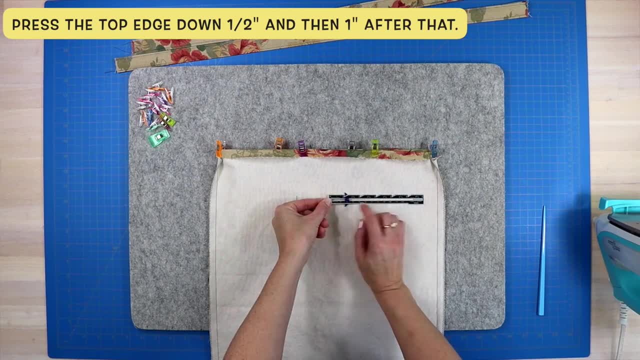 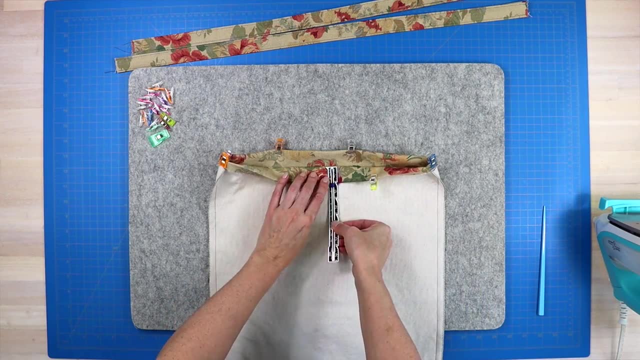 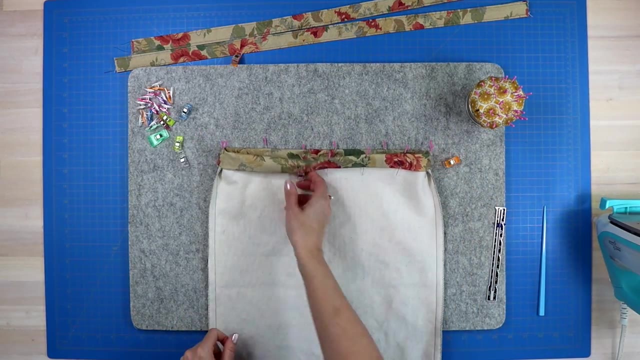 And now we need to do this same thing once again, except we are going to fold our top edge down a full inch Again. you'll use your measuring gauge to make sure that it's lining up the same around the entire outer edge. Just pin it in place. but this time I actually do like to use my long magic pins for this process. 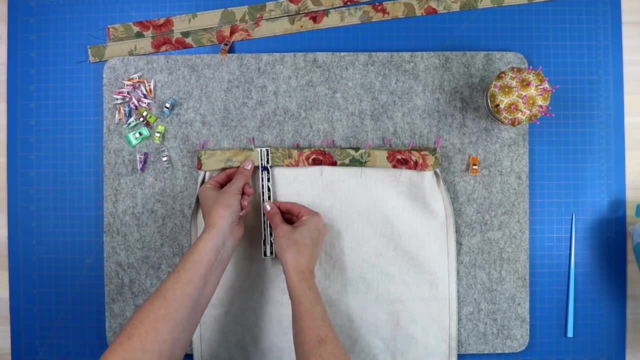 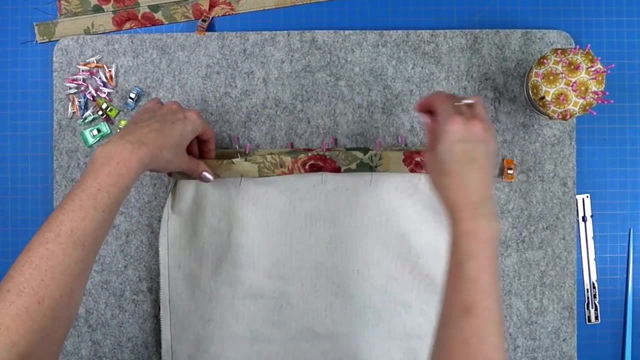 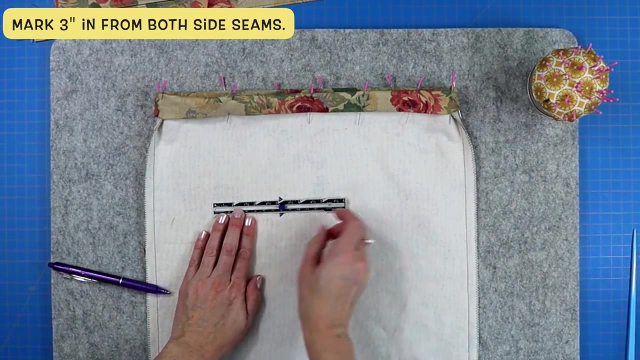 I find it's easier to hold everything in place that way. Once the entire top edge has been folded down at that one inch fold. now we need to measure in to figure out where our straps are going to lay. So you will measure from your outer seam in three inches and then 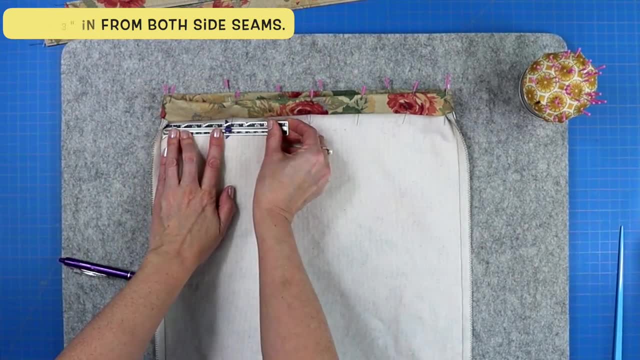 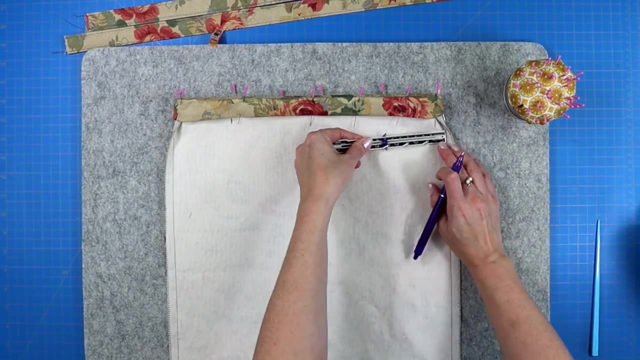 just draw a mark. You can use this with any marking pen you want, but if you want to get rid of those marks when you're done, make sure you're using a water soluble marking pen or a friction pen. I will have them linked in the description below. 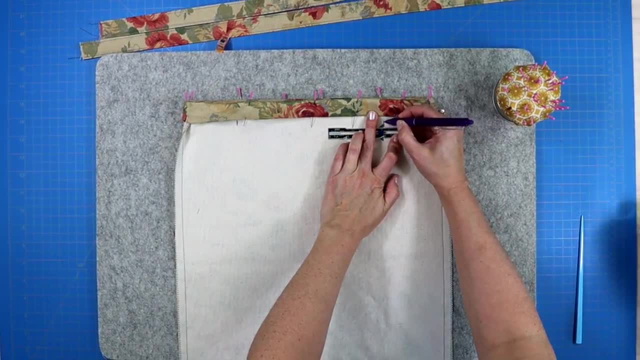 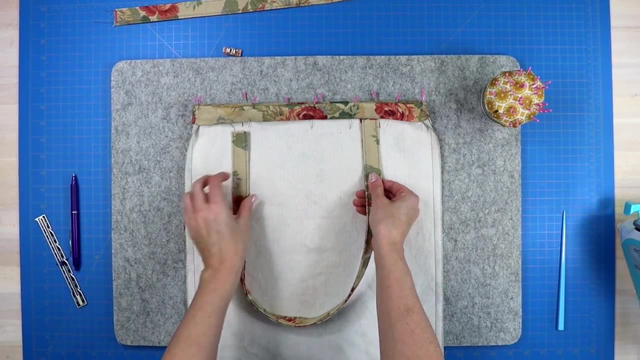 Along with my favorite sewing tool, that measuring gauge. It is the cheapest and most useful sewing tool that I have. Once you have those three inch marks on both sides, then you can tuck your straps in underneath that top fold and clip it in place. 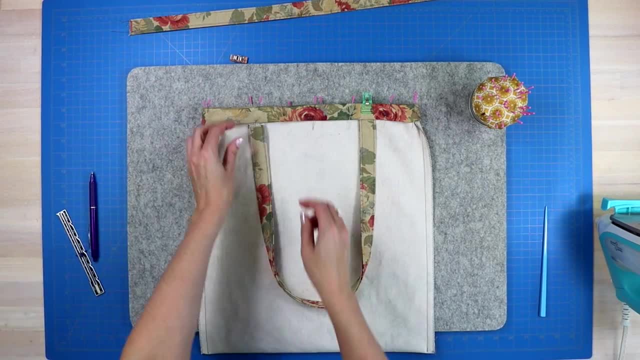 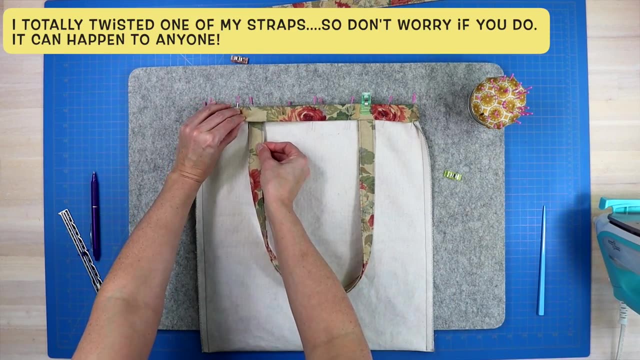 So the outer edge of your strap will line up with that three inch marked line that we made And, of course, make sure that your strap is not twisted as it goes around to the other side And then clip that end in place as well. Do this for both straps. 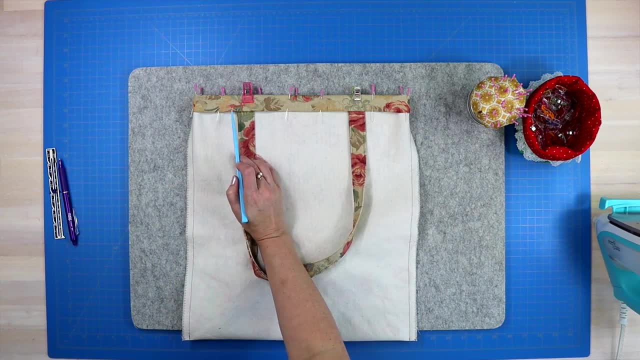 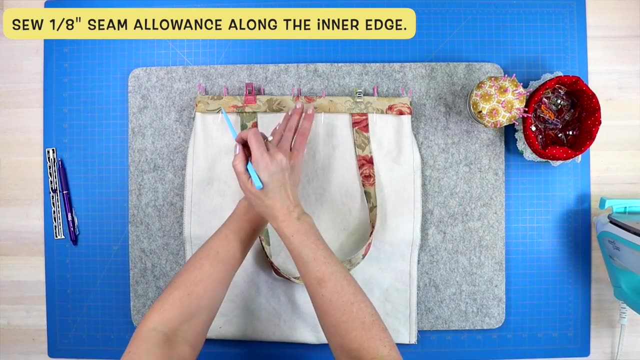 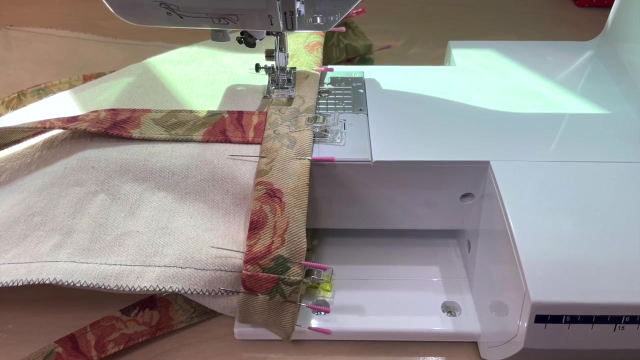 And now it's time to take this to your sewing machine and sew an eighth of an inch seam allowance around that inner fold all the way around the entire tote bag. The easiest way to do this is to remove that extra arm That is on your sewing machine, so that you can actually loop your tote bag around just a little bit easier.